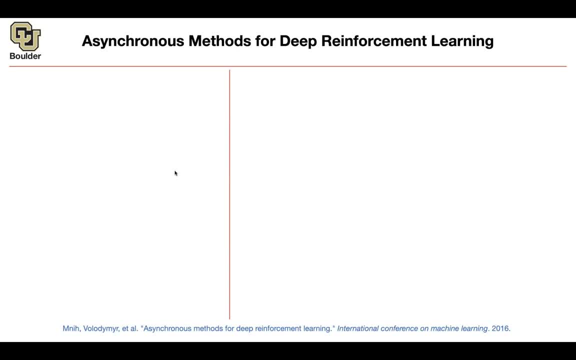 the idea You are still going to do policy gradients, but the idea here is, rather than having a single agent interacting with the environment, waiting for it to die or win the game or lose the game, we are going to spawn multiple agents to interact with the environment. 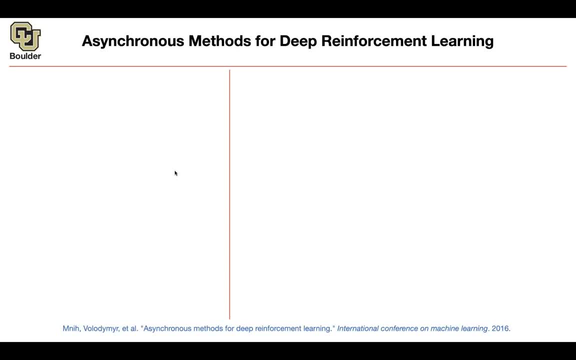 in parallel and then optimize over a shared set of policy. Let's see A quick recap of we just saw. you can have value-based model-free methods or policy-based model-free methods. For value-based model-free, you have a Q function that you're approximating by a neural network. That's going. 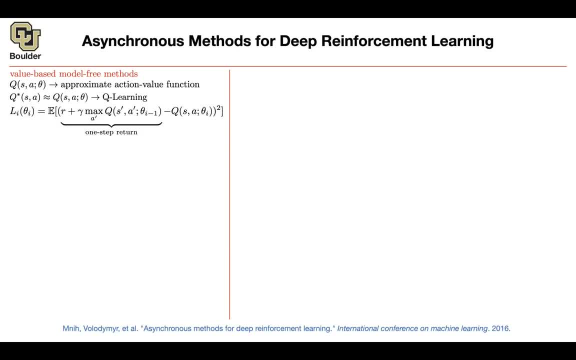 to be called Q learning or deep Q learning. We use the Bellman equation to turn a reinforcement learning problem into a supervised learning problem. The whole objective is learning this Q. And then we had one step return into the future, And this is coming from the Bellman equation. 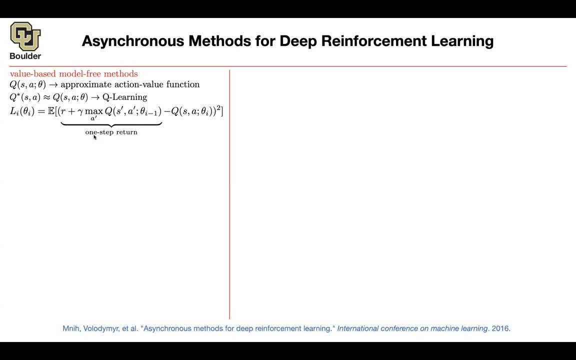 But we saw an example last session that the reward could be very sparse. Actually, you can get your reward at the end of the game, So you have to wait for a long time before you see any rewards. You can expand on this formula, this one step return and make it multi-step or N step. 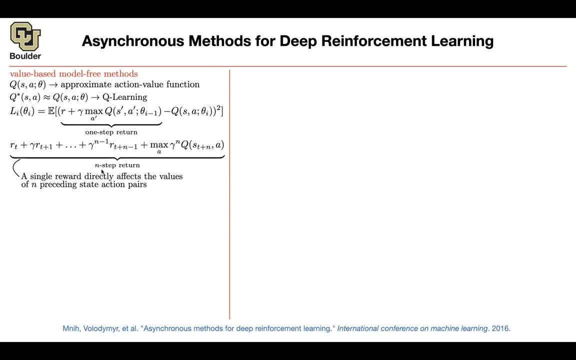 return. Why is it helpful? Because if you receive a reward, it's having an effect on N preceding state action pairs, So every single reward that you receive is going to correspond to multiple state action pairs. So it's giving you more feedback. That's one modification For policy-based model-free methods. 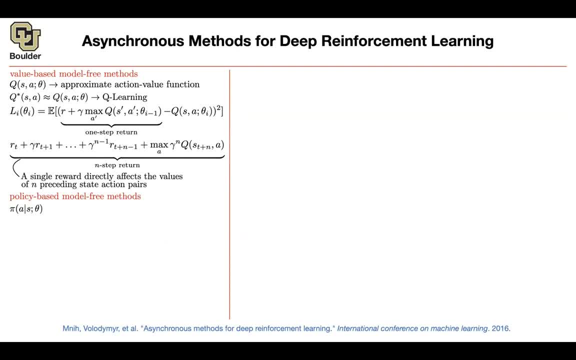 you model your policy, You say that I'm going to put a neural network on my policy, And then your objective function is no more coming from the Bellman equation. It's coming from maximizing your expected reward or minimizing your expected cost, expected future cost or 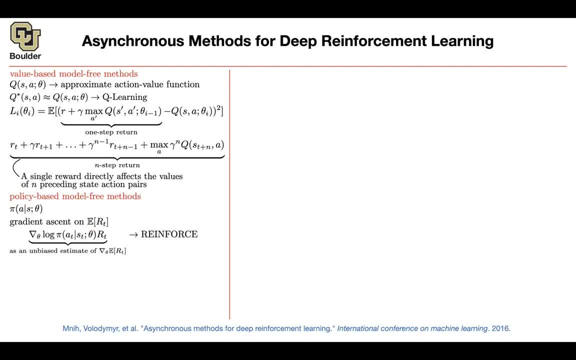 future reward. A simple version was reinforced algorithm, And basically what you're doing is coming up with a new algorithm, And then you're going to put a new algorithm, And then you're going to put an estimate of the gradient of your objective, But then, because this expectation is 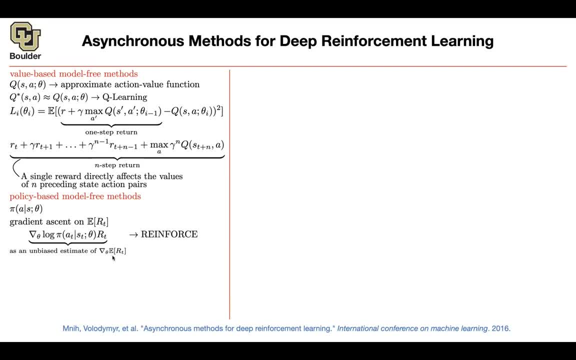 with respect to your policy. you have to do that trick, that the derivative of a function is the function itself times a derivative of the log of the function, And this is where the log is coming in and the expected value. you're dropping it because you're doing Monte Carlo. So this is an 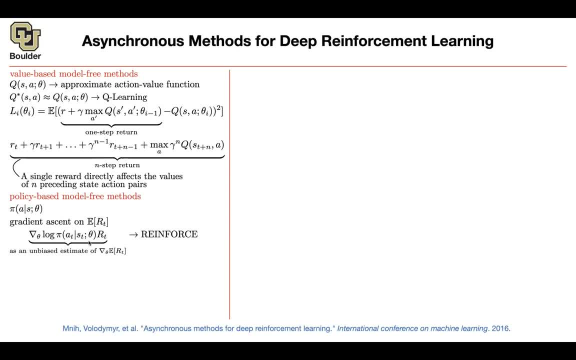 unbiased estimate of your gradient. But then we said this has a high variance. To reduce the variance, you're going to subtract the value of the gradient. So you're going to subtract the baseline. How good is your return compared to a baseline? This is still going to be an unbiased. 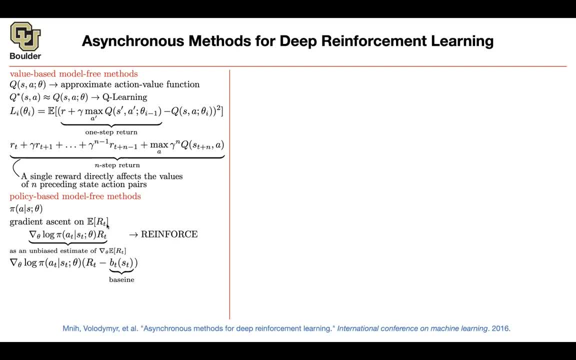 estimate of the gradient of your objective, but it has less variance compared to using RT only For the baseline. it could be any function that doesn't depend on your actions, So you can put any function here that doesn't depend on your actions. It can depend on the state, but it 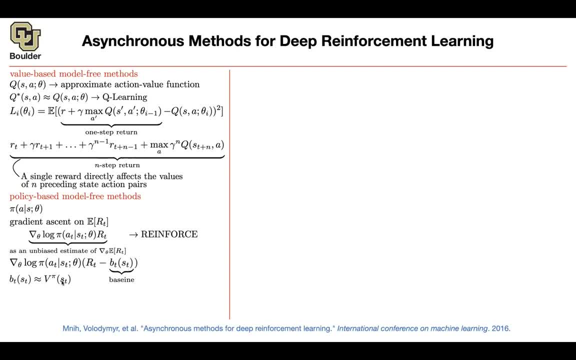 shouldn't depend on your actions. So, for instance, you can use your program. You can use your program on the average value, And this term here has a name: It's called advantage of action A in a state, S compared to the average action. So that's your advantage, the return. we know that you can. 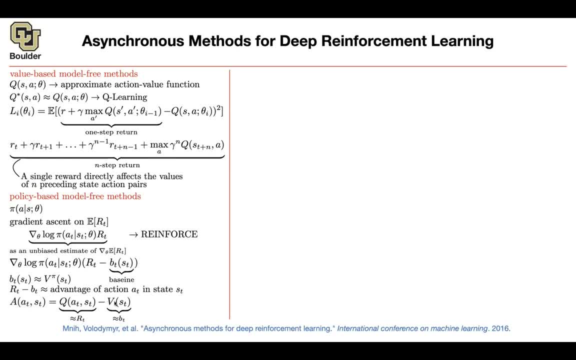 approximate it by your Q network, And this is the actual definition of the advantage that we saw last time. And V is just your BT. the framework we're going to cover today is called actor critique on your policy. So you're going to act based on your policy and then your B or your value is going. 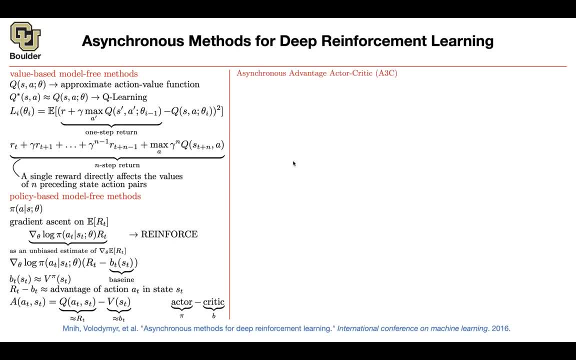 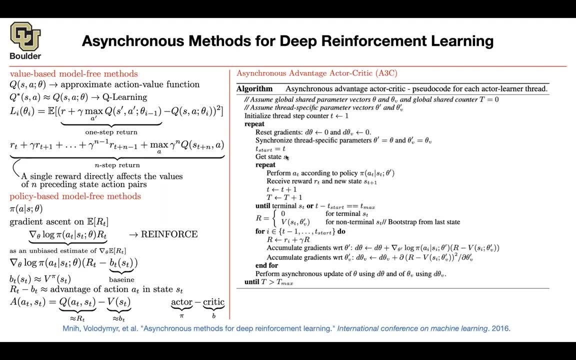 to criticize those actions. The idea was that you can spawn multiple actors in your environment and let them interact in parallel with your environment and let them asynchronously update their policy- actually a shared policy. So you're going to have a global, shared set of parameters. 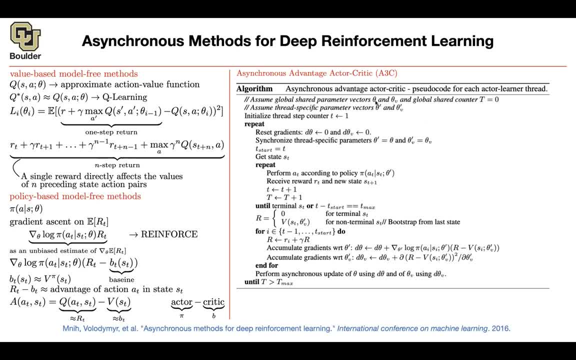 theta and theta V. Theta are for your actor, your policy, Theta V are for your value. And then you don't want to go forever. You want your algorithm to stop at some point, let's say at T max. So you're going to set capital T to be a counter, and then you start from zero. 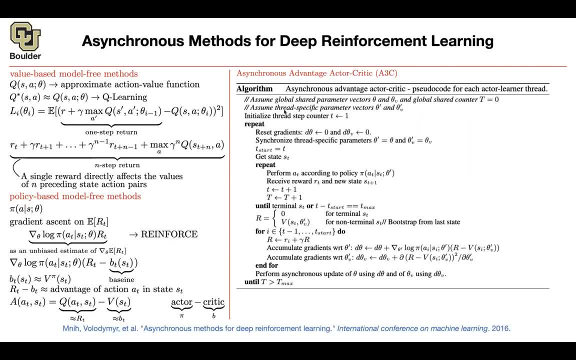 And then you're going to have: each thread on your computer is going to be an actor, It's going to be an agent And each one they're going to have their own parameters for their policy And for their value. And then each one of those threads is going to have their own. 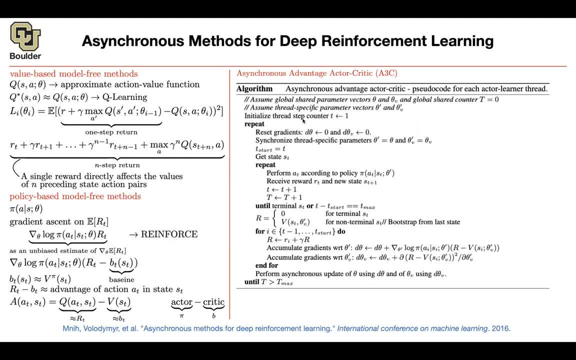 respective step counter. They're going to live in your environment for a while and then die or win or lose, and collect rewards or get punished. So they're going to learn on their own. Initially, you set their gradients to be zero. They are going to inherit from the shared policy. 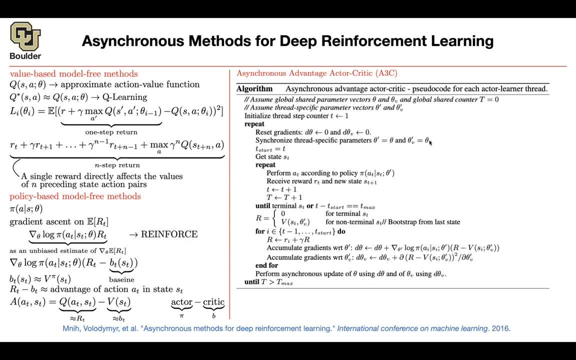 and the shared value. So you're just going to inherit some parameters from your the global environment, And initially T is one, So T start is going to be one. You get the state at the start And then you're going to live in that environment for a while. 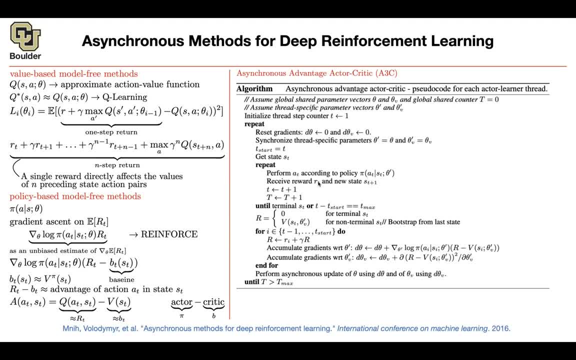 You're going to take actions based on this policy. You're going to receive rewards. go to the next step and then increase your counter. Either you are in the terminal state or you have been living in that environment for too long, And then we are going to kill you. 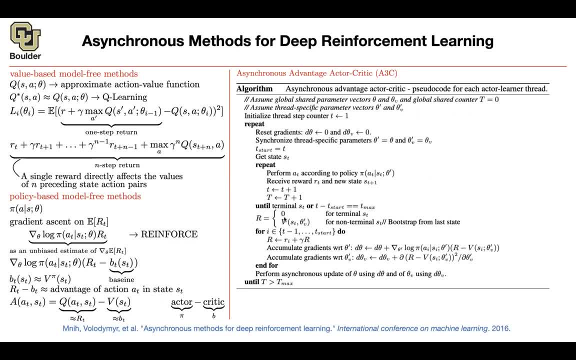 kill that threat. If it is a terminal state, there is nothing going to happen in the future. No reward, no nothing. So that's going to be a return of zero. Otherwise, this is where you're going to call your value, to have an estimate for the type of rewards that you're going to collect if you are to follow this. 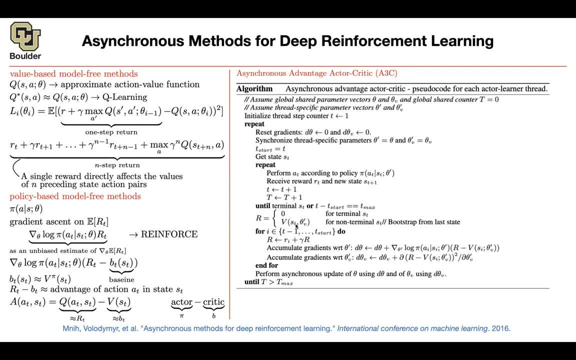 policy. So that's just an estimate for what's going to happen in the future If this is a non-terminal state And then you're going to go backwards. This might be a little bit confusing, But this is exactly the math that you see here. 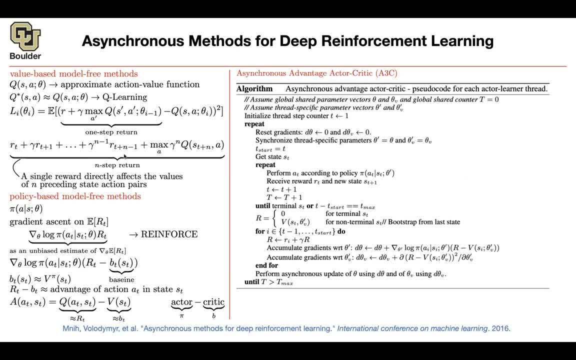 So what you're computing is this guy, this term here, but you're computing it backward. You first compute R and then you multiply it by a gamma and then add the previous guy, And then you keep iterating and you go backward. You compute this term backward. 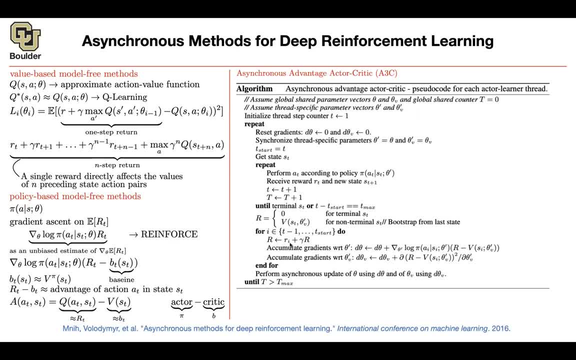 The next step. this guy is going to become gamma, squared gamma Ri plus Ri minus one, And then you compute your R. You're going to use R in two fashions. This is your labels. You're going to use them to update your value, which is very similar to what you're doing. 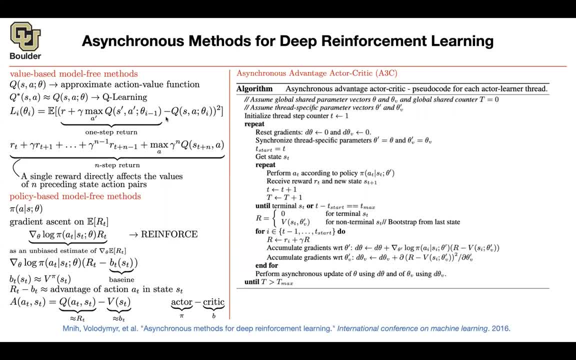 here. That's your loss function and you're doing mean squared error. So that's your mean squared error. And then the other guy is coming from this term. here, the reinforced algorithm. It's going to be R minus the baseline times, the gradient of your log of the policy. 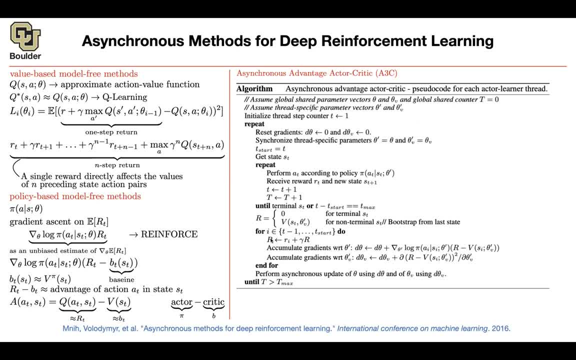 Each one is going to do their own job. As soon as their iteration is done, They're going to update the baseline, They're going to update the shared parameters asynchronously and then either move to the next step or die, or something is going to happen to them to that threat. 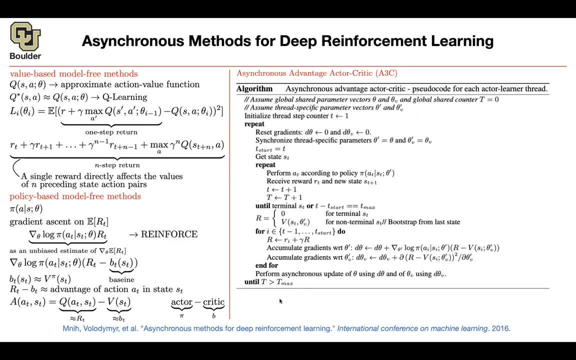 So you're learning in parallel and collecting a lot of data. A little bit more details about this R. What you're writing here is basically nothing but the advantage and the advantage. you are computing it by V of ST, which is this term here. 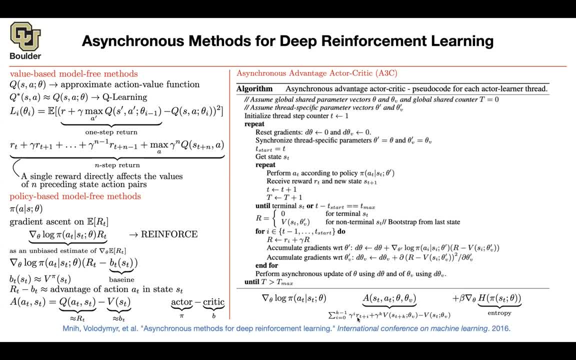 And that R is going to end up being the summation of R. Okay, So you're going to get the estimation of your returns plus an estimate of the future, which is coming from the future. What's going to happen if you don't actually simulate, but estimate? what's going to happen?